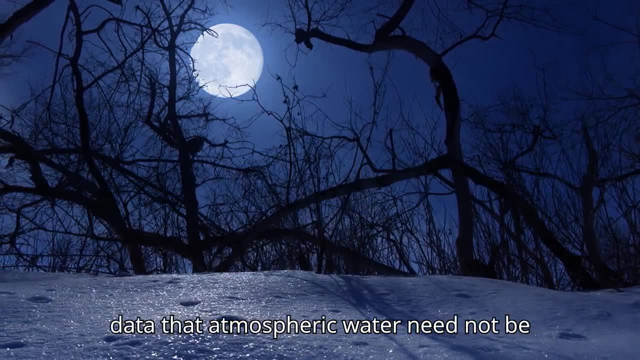 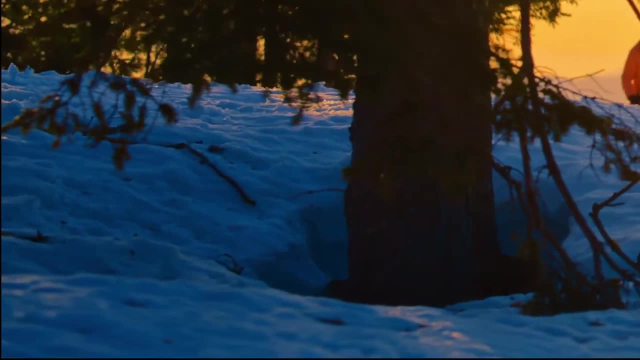 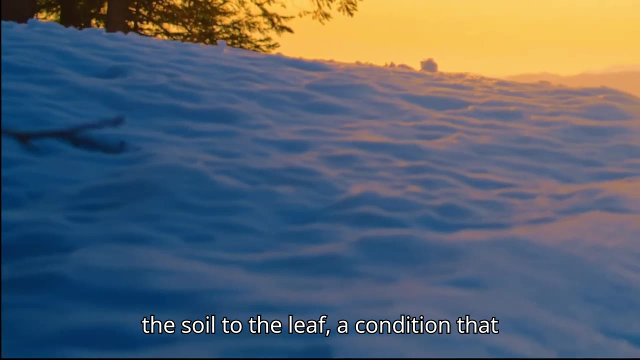 It can be concluded from the observation of the data that atmospheric water need not be so dry to pull the water from the plants through the soil by the roots. Even a drop of 1% in RH is sufficient to raise sap from the soil to the leaf, a condition that always 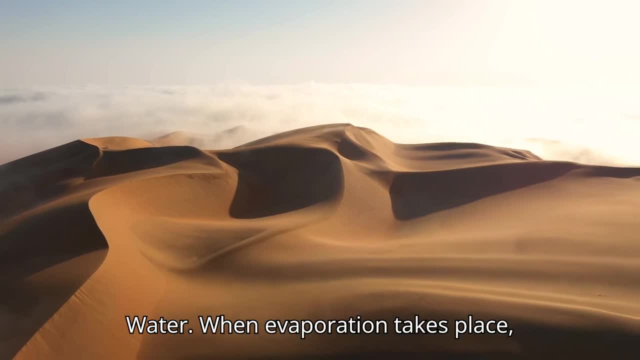 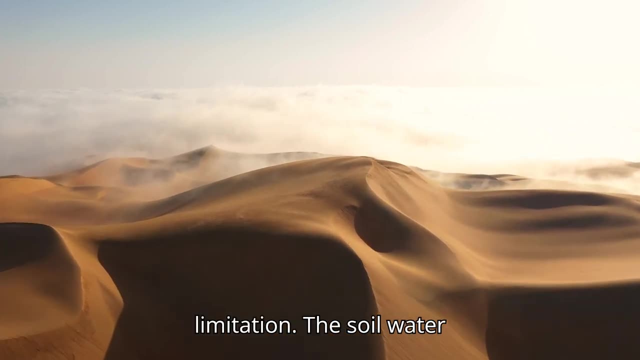 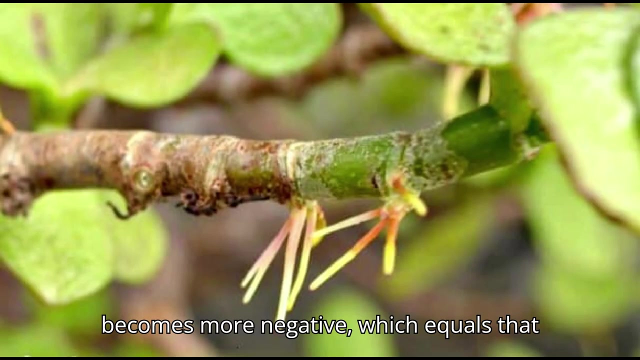 prevails in the atmosphere: Water. when evaporation takes place, water from the soil also evaporates and dryness of soil occurs, which has a limitation. The soil water becomes thinner and water potential becomes more negative, which equals that of the root, so no further absorption takes place. 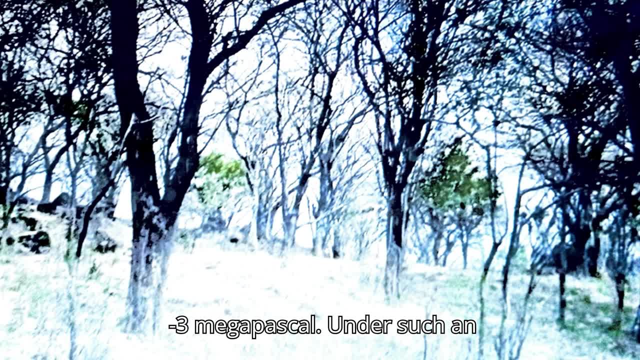 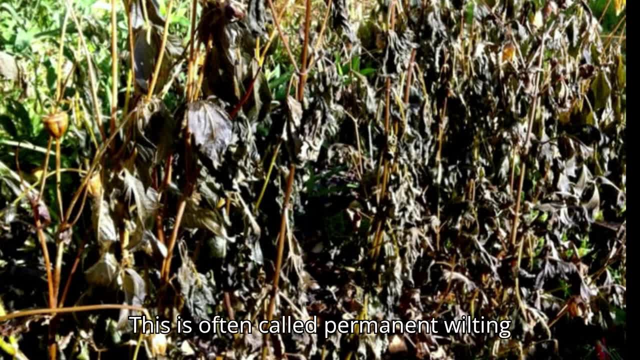 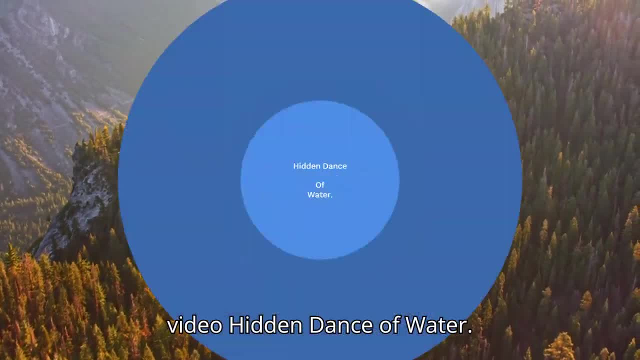 The value is approximately minus 3 MPa. under such an equilibrium, water is lost from the stem and leads to the wilting of leaves. This is often called permanent wilting percentage, which is dependent on the type of soil. See the video: Hidden Dance of Water. 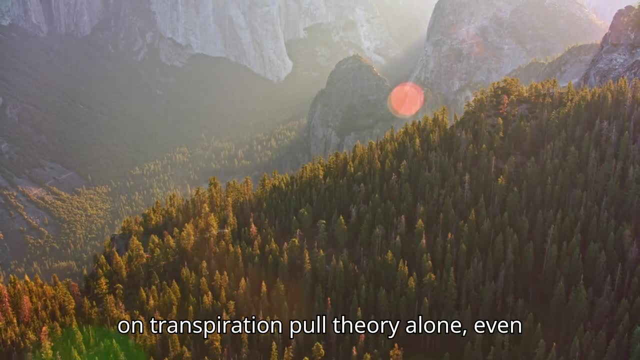 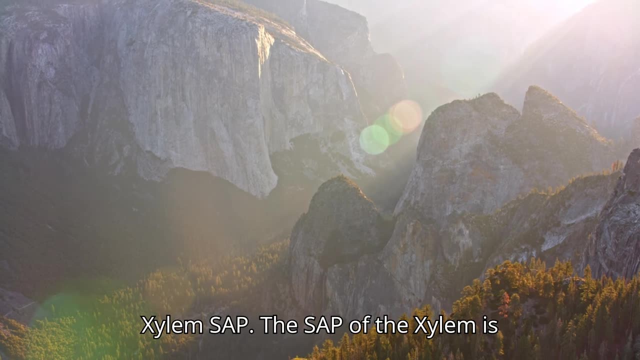 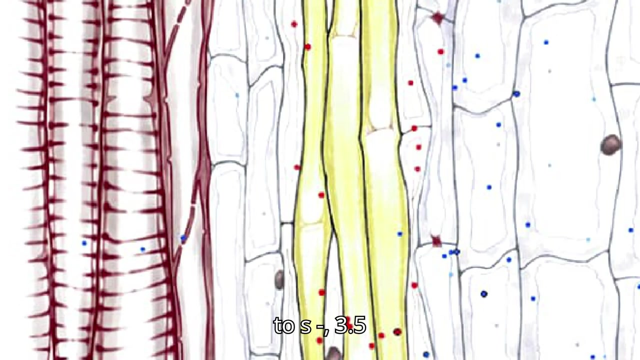 This answers questions 1 and 2, based on transpiration pull theory alone, even if other conditions work against it. Xylem SAP, the sap of the xylem, is very dilute, while the water potential in parenchyma cells is 0.3 to 3 to S-3.5 MPa. 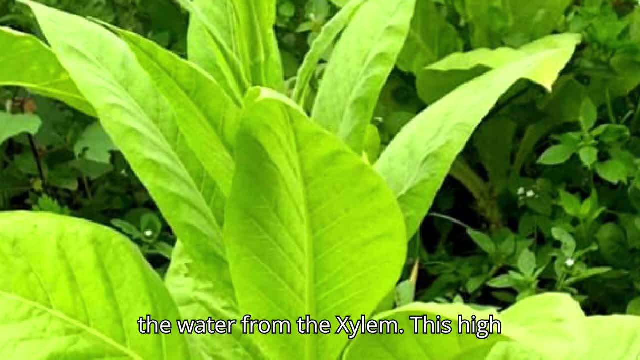 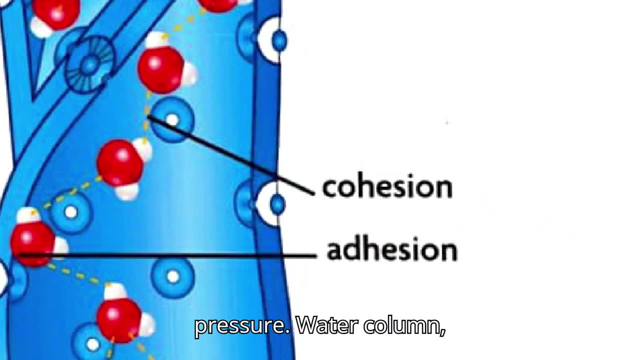 which is sufficient to pull the water from the xylem. This high pressure in the leaves is due to combined effect of turgor pressure and osmotic pressure. Water column. another factor that maintains the water column in the xylem is dependent on: 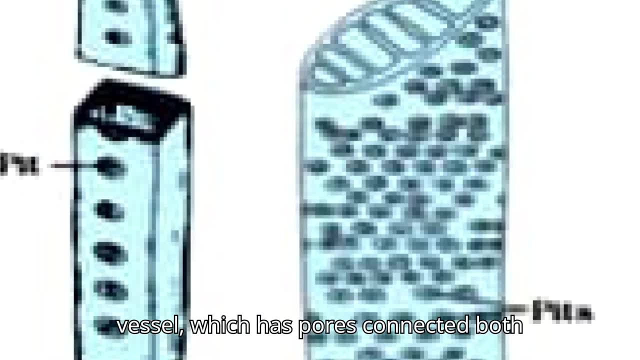 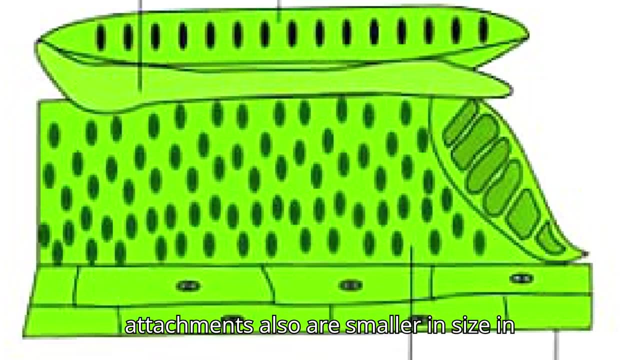 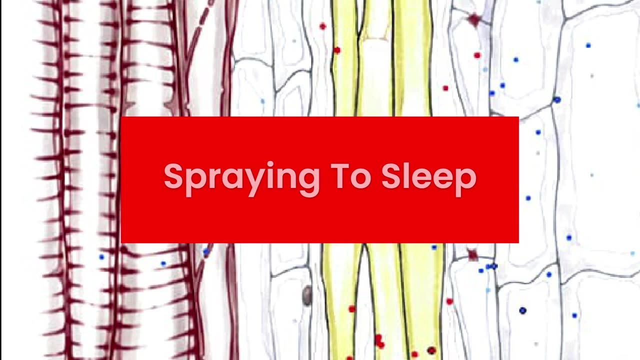 The structure of the xylem tracheid and vessel, which has pores connected both apically and laterally. zigzag attachments also are smaller in size in tall trees when compared to small plants. Watch the video: Spraying to Sleep. Lateral pores in the tracheids and vessels of the xylem are responsible for maintaining water columns. 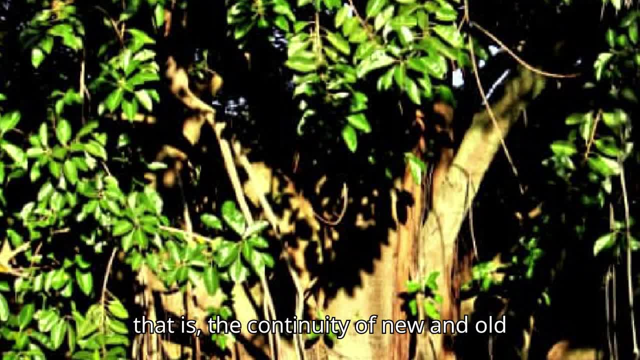 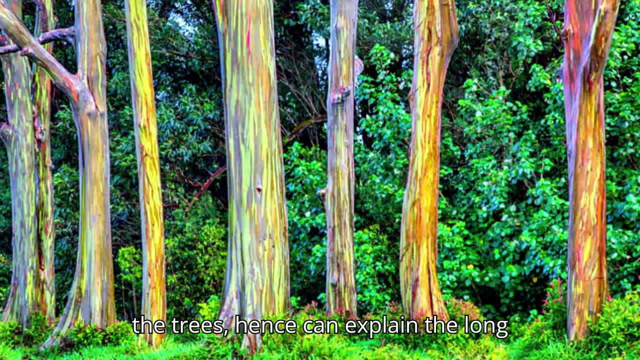 despite the annual leaf shedding and wood formation. that is the continuity of new and old xylem after the onset of spring season in the trees. hence can explain the long survival of woody plants and rapid rate of water requirement with the onset of new leaves.